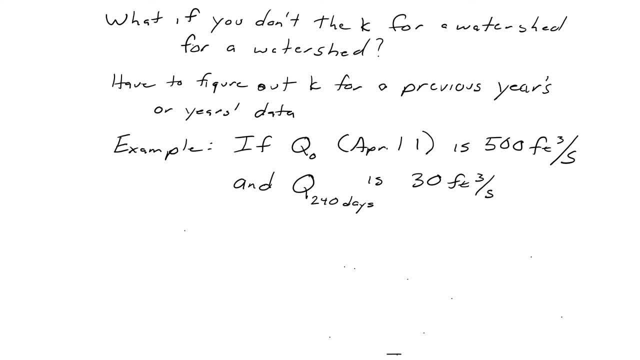 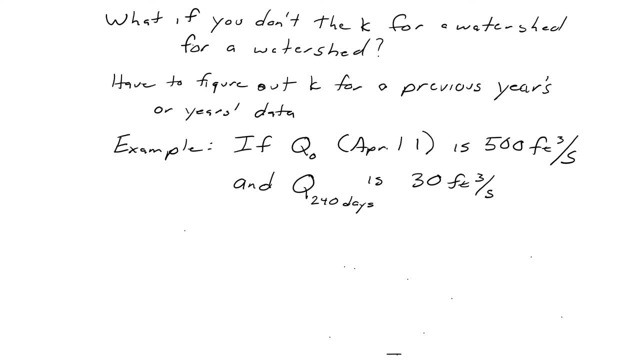 stream. Okay, so it's 500 cubic feet per second. on April 1st, Eight months later, so much groundwater has been transferred from these alluvial aquifers into the stream. Now we're down to 30 cubic feet per second. What we can do is take our 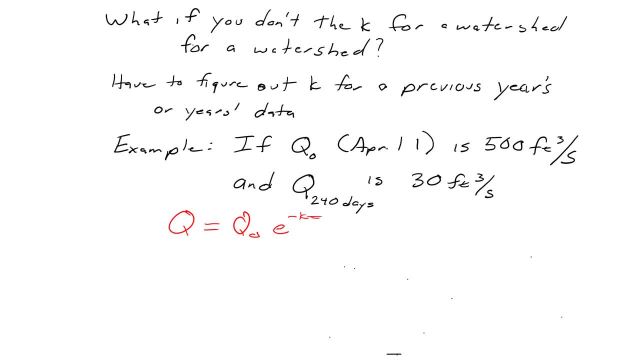 base flow recession. equation Q equals Q-naught e to the negative kt. we actually have everything now but k and we can now solve for k. We did this last week. I think it's worth going through again. So if we just put down what we know so far, 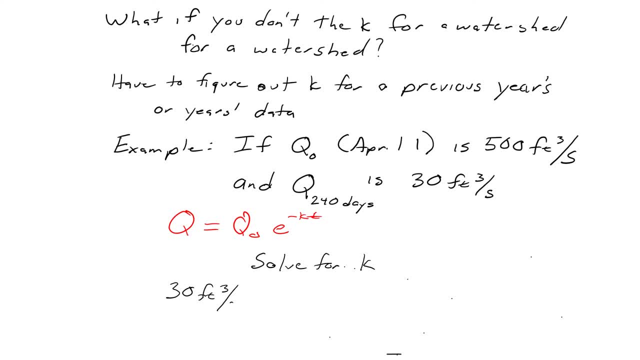 we know that that 240 days in we have a discharge of 30 cubic feet per second. We started out with an initial discharge of 500 cubic feet per second. e to negative k, which we don't know, but we know t is 240 days. 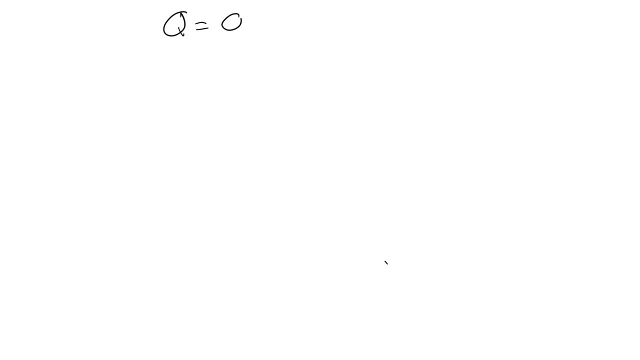 So what we can do is we can rearrange the equation. We start with q equals q naught e to the negative k t. We're going to try to isolate down to k so we can get q over. q naught equals e to the negative k t. Last week we talked about the way you 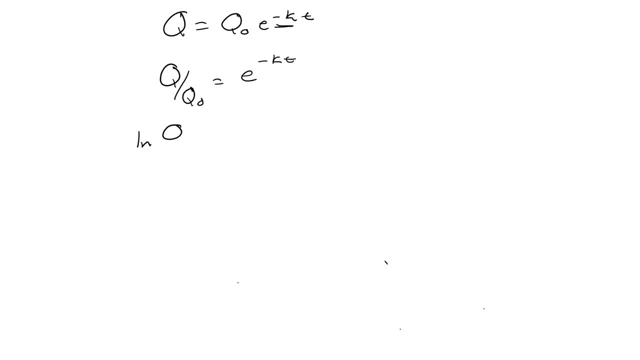 get rid of the e. the exponent in this is is to multiply both sides by your natural log, And when you do that, ln times e is 1, and you're left with your exponents. So we can just put this in: ln, 30 cubic feet per second. 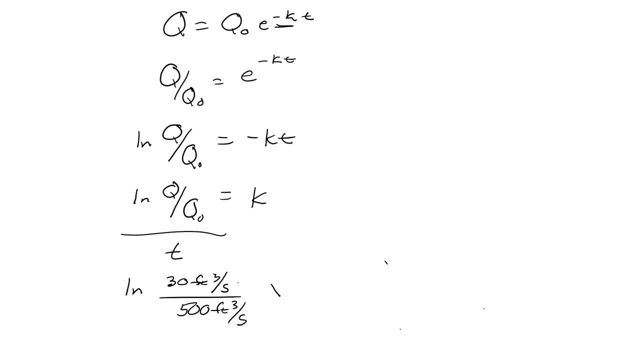 over 500 cubic feet per second. So we can just put this in: ln. 30 cubic feet per second times 1 over 240 days. The units cancel out. That's going to equal your k And if you multiply this out you end up with a k. 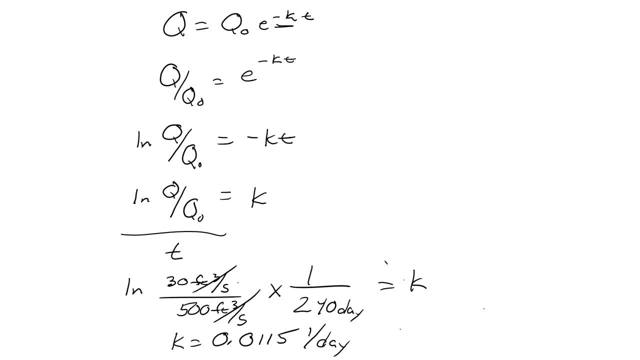 that equals 0.015.. And the units are 1 over day. We went through it a little more detailed last week so you can look back at your notes to see some of these additional steps. OK, so that's your k. 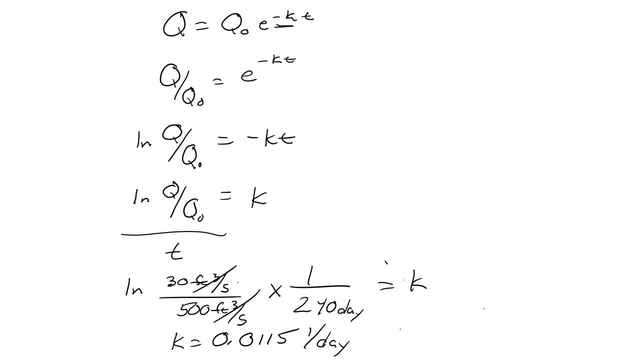 That's how you take this equation, work it sort of backwards with the previous year's data and get the k for the watershed, And again all these different watersheds are going to have different k values depending on what the land cover is like. 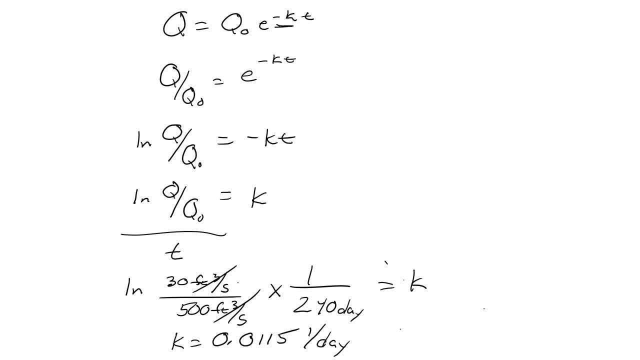 how big the watershed is, how big the alluvial aquifer is, how porous and permeable the alluvial aquifers are. So it's all this physical stuff that's going on in the basin that's going to determine this k. 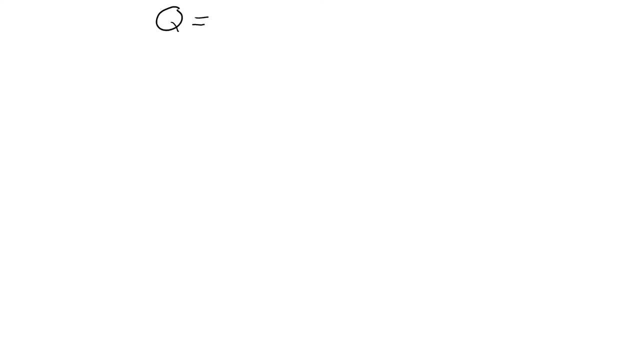 OK, so now let's use this equation. I'm going to put it back up, And that's where we ended last week: q equals q0 e to the negative kt, So we're going to keep using this. So your next. 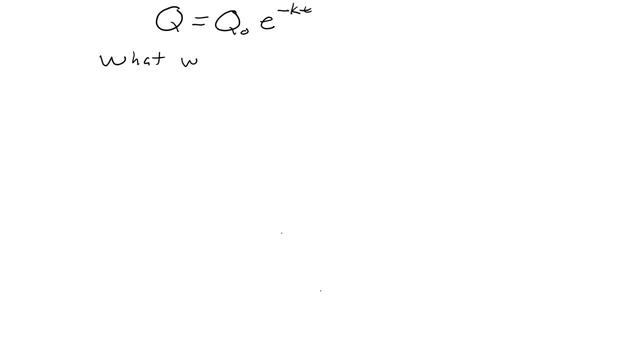 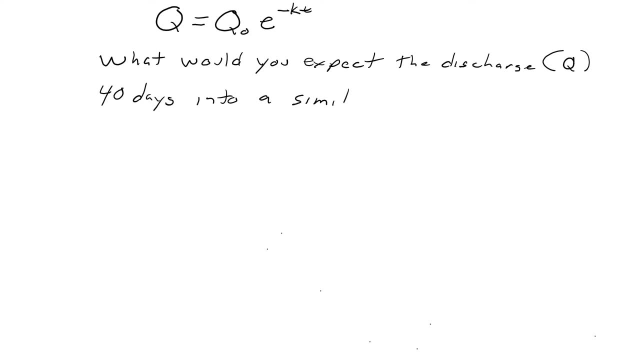 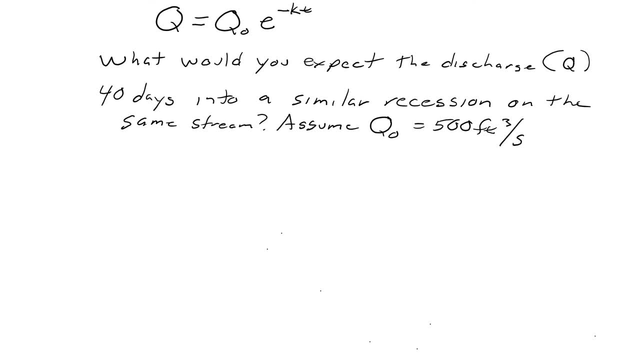 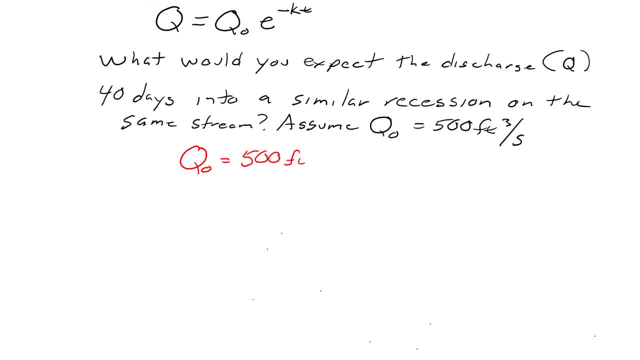 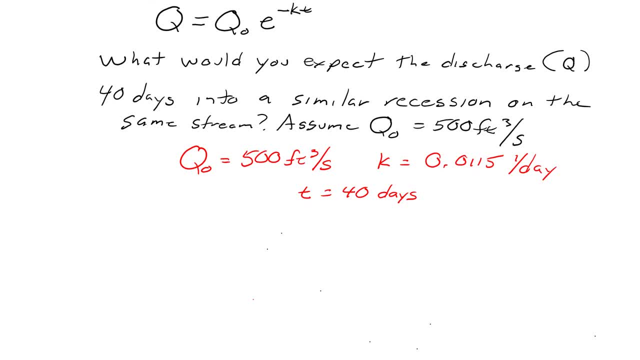 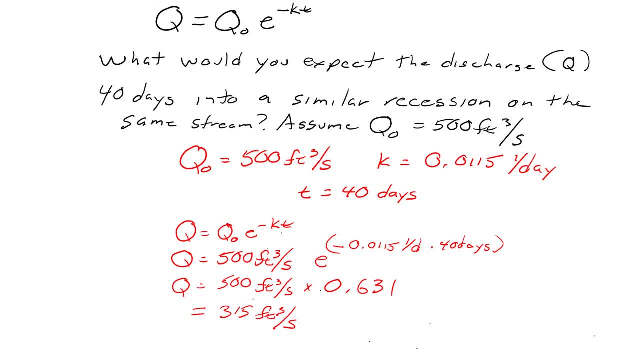 greater than 500, you did it wrong. Okay, It's only a month into the recession, so if you think about the curves, you can kind of think about what your ballpark might be. It's going to be less than 500.. Obviously more than 0. 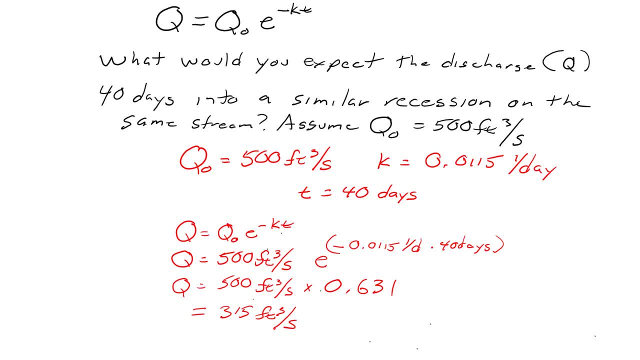 This isn't very far along, so it's probably closer to 500 than it is to 0, but that depends on your k value. Now, one thing that didn't come up with this example that really pay attention to in future examples: this term, right here. 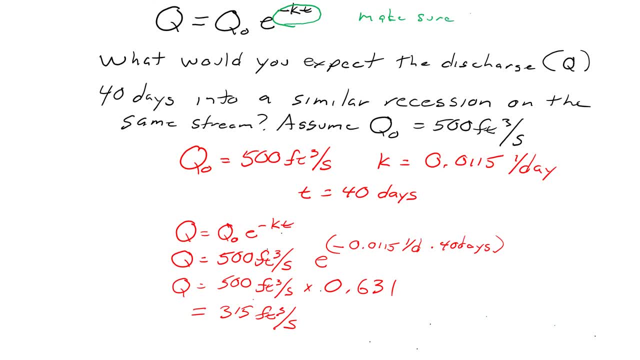 negative kt. make sure the k and t cancel out in terms of units. In other words, they have to be days- 1 over days, hours, 1 over hours. days need to be units that cancel out. So make sure those two cancel out in terms of units. 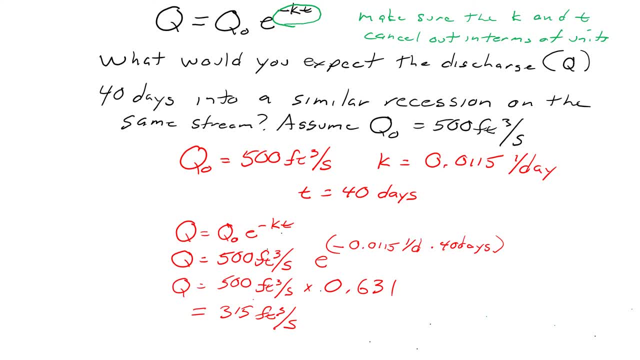 In this case, our k is in 1 over days, our time is in days, So they're going to cancel out. that's great. So when you take your k, negative .0, 1,, 1,, 5,. 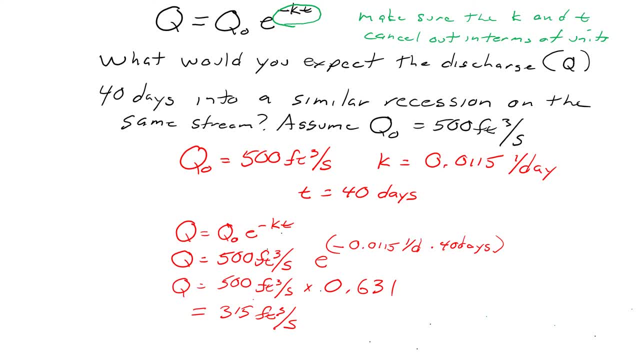 multiply it by 40 days e to that quantity should give you 0.631.. A little more than a half times 500 should give you a little more than half of 500.. A little more than 250, and in this case you get 315.. 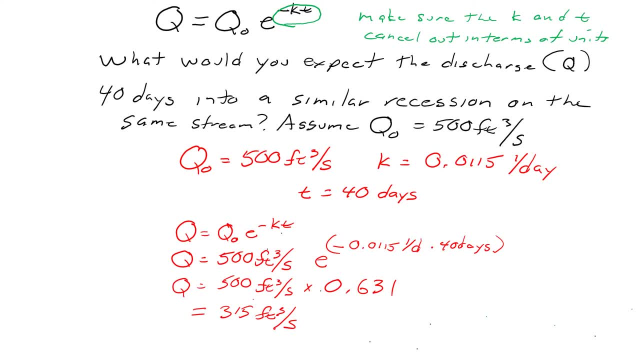 Alright, any questions on that? Any problems doing the exponents? Okay, What are you getting for an answer? 274.. Anybody else get that? I just want to make sure I didn't do the math. You got 315?. 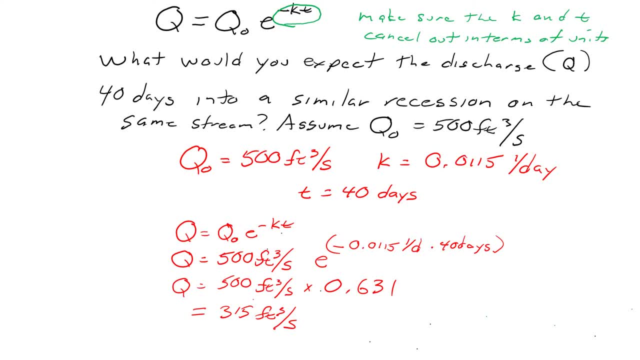 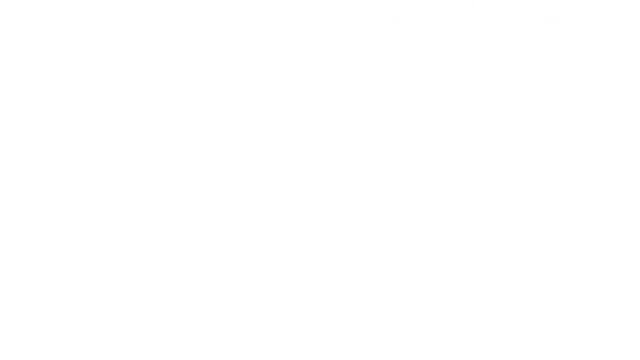 Alright, you got .0, 1, 1, 5? Times 40?? You got .1, 1, 5?? Okay, It will make a little difference. yeah, Okay, So just the typing in error. 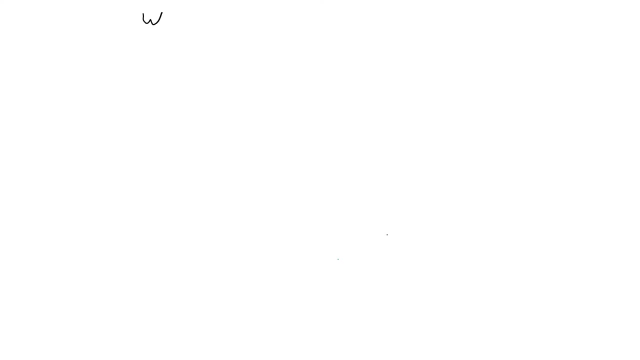 That's good, Okay. So another question, just to give you a chance to play around with this a little bit: What if next year's reset? what if a recession lasts 9 months, So the snow melt takes a month longer to get going next year? 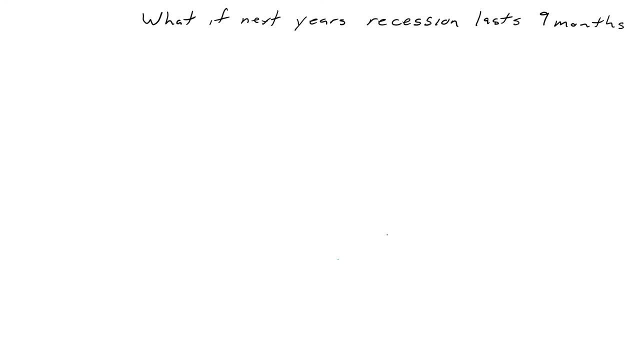 For whatever reason- different weather, whatever- So you have a slightly longer recession. What I want to know is: what would the discharge be at the end of that? nine months? And you can just assume 30 days per month to make the math a little easier. 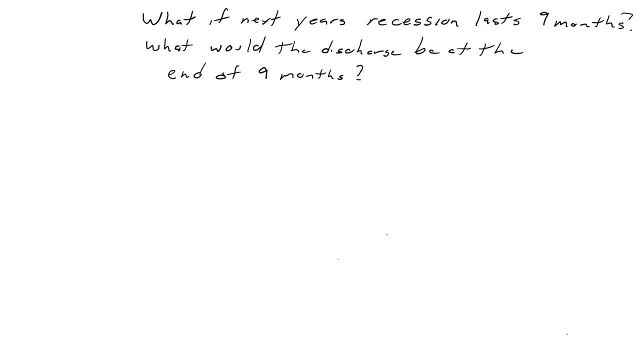 You can just assume 30 days per month to make the math a little easier. Thank you, Thank you, Thank you. Okay, if you run the math through, you're doing nine months where this is gradually tailing off and you end up with a pretty low discharge: 22.4 cubic feet per second. 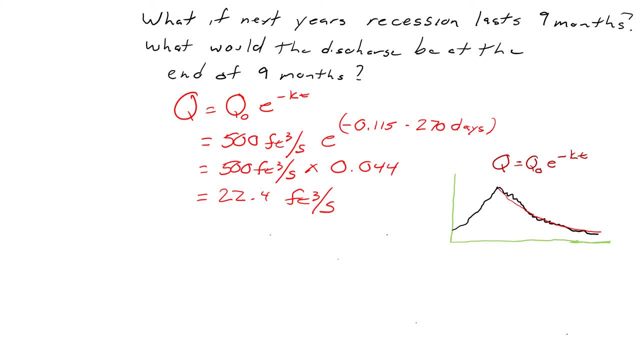 I bet if you went down to the Poudre River today, it's actually pretty similar to that. It's probably 20, 30 cubic feet per second. That's a trickle in a stream that size. Now, remember when you see equations like this: 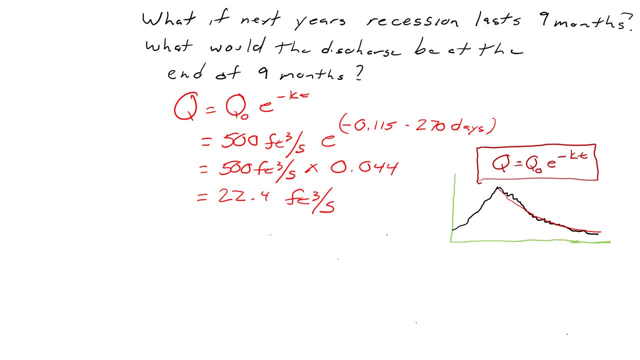 designed to mimic nature. these are just best fit. They're best approximations. Okay, They have some assumptions built in. You see the shape of this red line. The red line sort of represents what would happen if you ran the times from the. 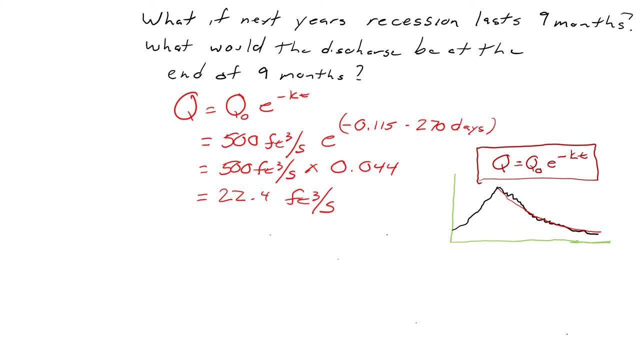 beginning to the very end. Is it ever going to hit zero? do you think You guys have seen mathematical expressions that have that sort of exponential tail off right, Asymptotic expressions? what don't they ever hit? They never hit zero, do they? 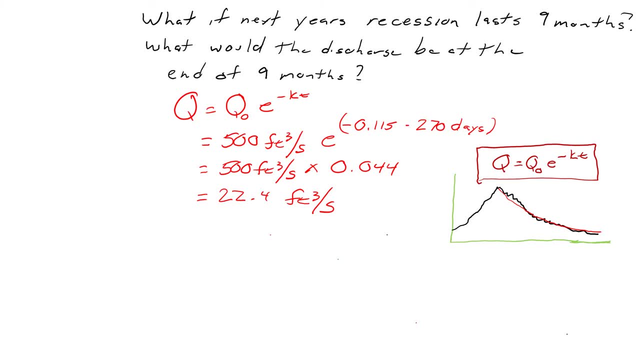 So mathematically you're never going to get zero or below zero with this Doesn't matter. you could put in 10 billion years. okay, You're not going to get zero. But think about out in nature, Do you think your? 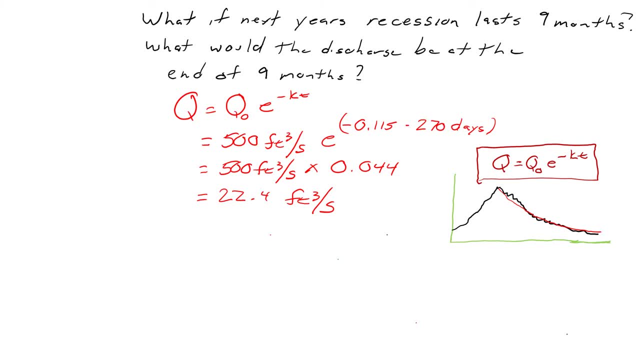 alluvial aquifers. if they're never replenished with any water, are they eventually going to run out? Yeah, So these equations have limits. okay, So that's just one thing you should always know is that these are approximations. 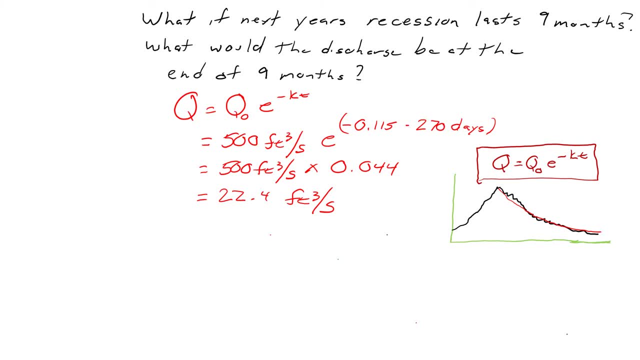 They have limits. I mean, clearly, this mathematical expression is never going to hit zero. That's what this decay function does, If it approaches zero but never hits zero, but never quite touches. But in real life, yeah, It could certainly be a case where your aquifer could just run completely dry. 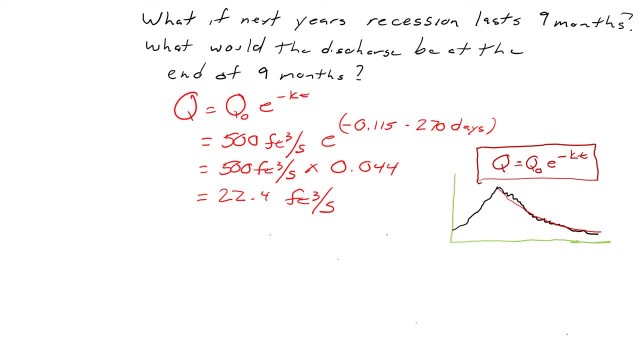 Okay, So just sort of keep that in mind as you work with these mathematical expressions. Okay, Any questions? Okay, That's, I think, about all we're going to do with base flow recession. for now, I have another comment. 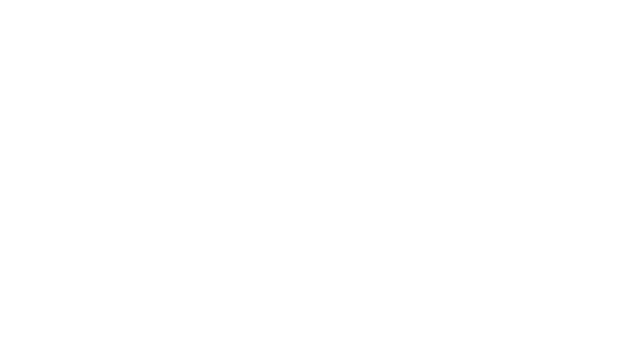 I have another concept for you that you may have seen in other classes. We're going to use it here for groundwater, And if you've had hydrology, you probably saw this. It's called the hydrologic equation And it's simple. 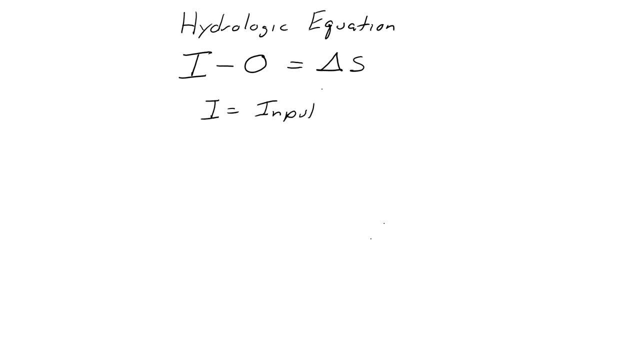 So I'm going to do a little math and explain a little math, And I'm afraid that I haven't put together the truth yet. Looks like I need to improve, So I will pause the. and this works for any hydrologic system, and when I'm talking about a system, I 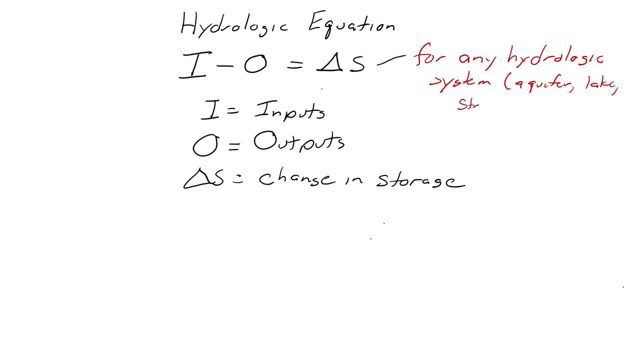 could be talking about something like an aquifer, a lake, a stream, a glacier, some sort of physical body that holds water. okay, that's what we mean by a hydrologic system. let me give you an example. let's say we have a reservoir fed by a river, and then the dam can be released into a downstream portion of 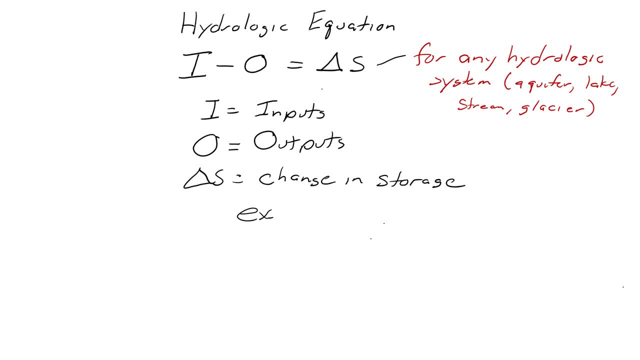 the same river. so you have a river, you stick a dam on it and the dam holds back water as a reservoir. okay, so the reservoir is going to be the system of sun into the현. okay, so imagine Estis Lake, imagine, imagine any impoundment that's held back by a dam. 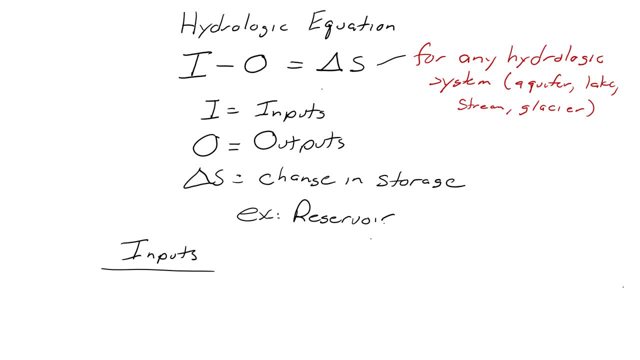 what could be some inputs to that reservoir? where could the reservoir get some water runoff off? Okay, let's think about that. We could have runoff directly into the reservoir, right, Just off. Think about sort of the edges of the reservoir, right, If it rains, water can just. 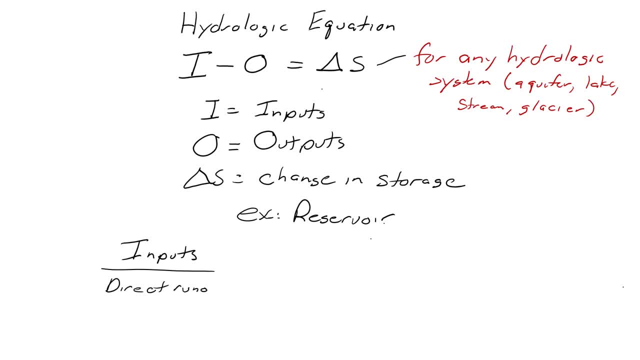 run right in there, right? Okay, so you could have direct runoff into the reservoir, But you could also have runoff going into a stream that then feeds into the reservoir, right? So we'll list that as something a little different. We'll do. 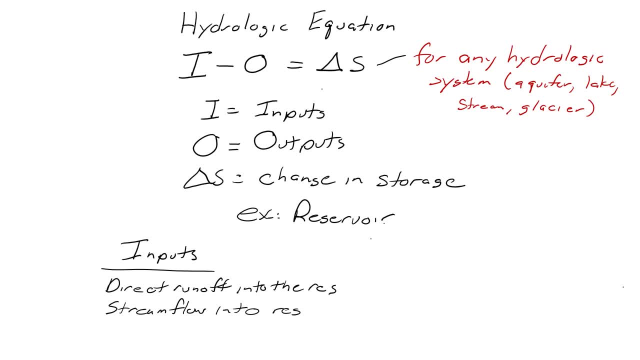 stream flow into the reservoir. How else might the reservoir get some water Raining right on the reservoir, right? So precip onto the reservoir. Okay, so we got stream flow, We got a little bit of runoff, We got rainfall landing on it. 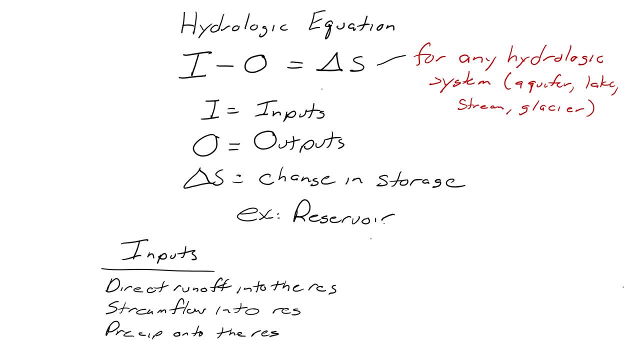 Think of anything else: Groundwater moving in. There might be some groundwater moving in. Okay, those are all the ones that I thought of. What about outputs? How might the reservoir lose water? Okay, outflow, stream out what they let loose and downstream. 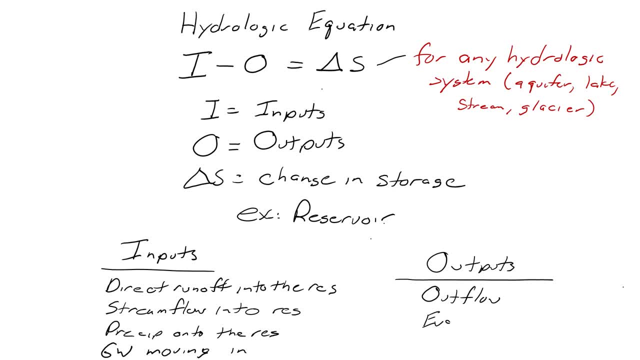 We'll just call that outflow, Stream flow. You said evaporation. Can you give me anything else? Groundwater might be moving out. You don't really know. I haven't given you enough information, but we could have groundwater out. 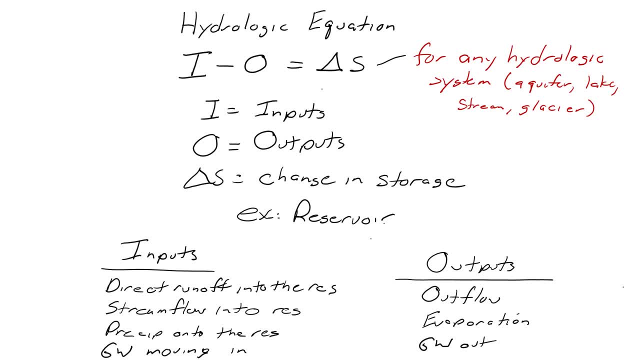 What if your inputs are greater than your outputs? How's the reservoir going to respond? It's going to have more water, right? So in this case, if your input is greater than your output, you're going to have. let me do this. 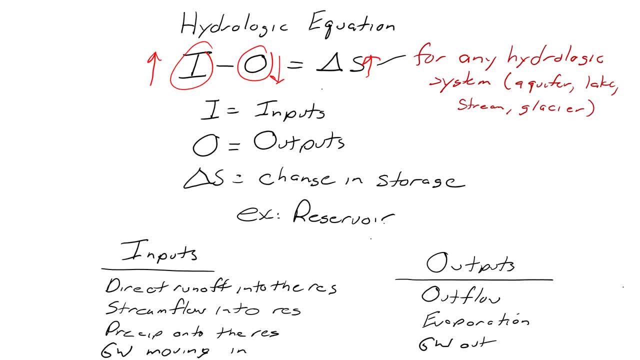 input greater than your output, your storage is going to increase, right? If it's the opposite, if your output is greater than your input, you might have a negative, negative change in storage and your level will go down. So what we do in hydrology is we try to 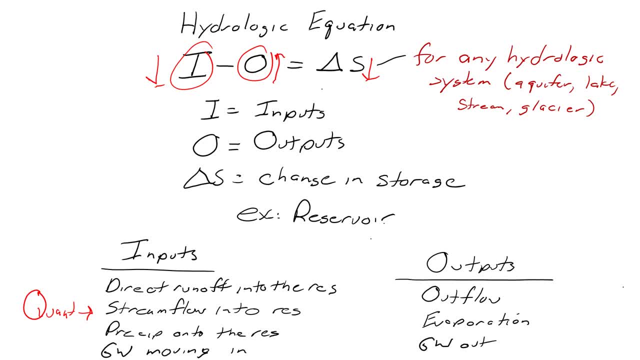 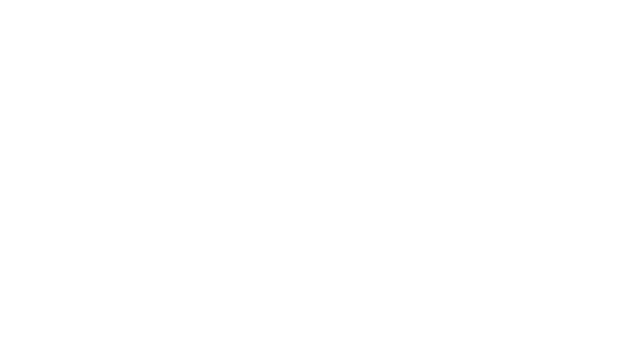 quantify all of these things as best we can, And that will tell us how our systems are going to respond in the future And what I want to do. let's see if I can get this to work. I'm not sure I can get this to work. 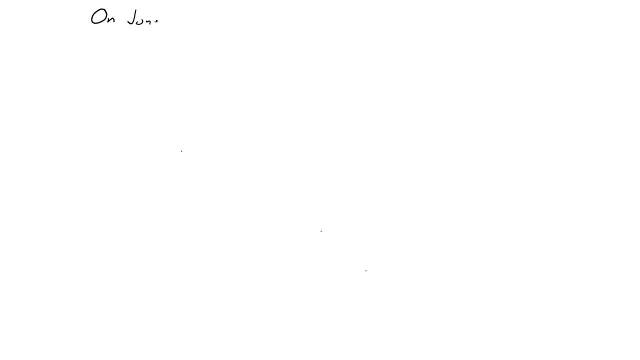 All right, So I'm just going to write this out, So I'm going to give you a problem here. So on June 1st the water in 140 acre it's going to increase. it's going to increase reservoir. 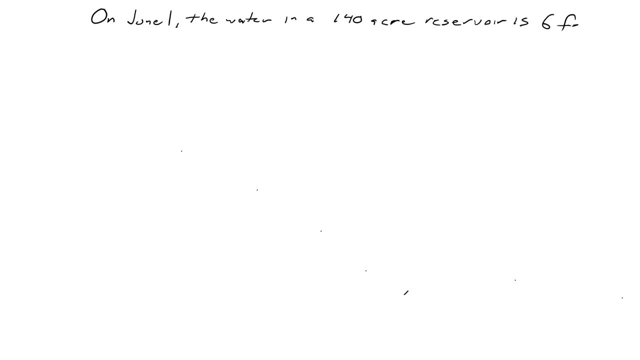 is six feet below the dam spillway, Or, in simple terms, that's the top of the dam, The maximum level that your water can reach in your dam. okay, All right, so it's six feet below the top on June 1st. 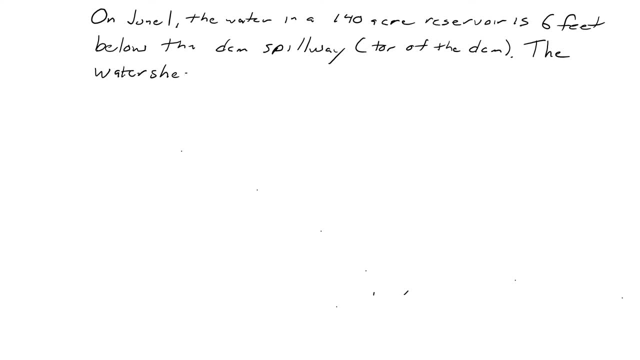 All right, let me give you some information about the area. The watershed that feeds this reservoir is 9,000 acres, And that does not include the reservoir. So you've got. I'll try to draw a picture out here in a minute. 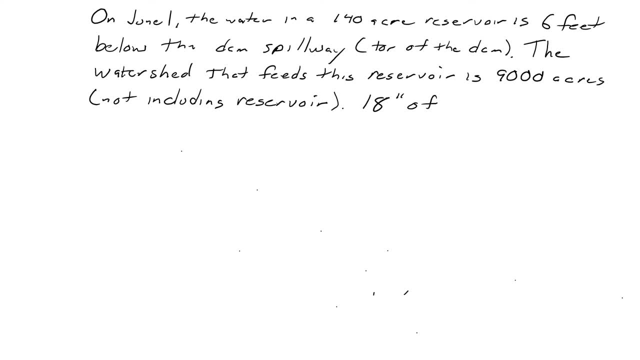 All right. so 18 inches of rainfall on the watershed and reservoir over the next 180 days. So over the next six months, a foot and a half of rain falls on the watershed and on the reservoir as well. The area is also subject. 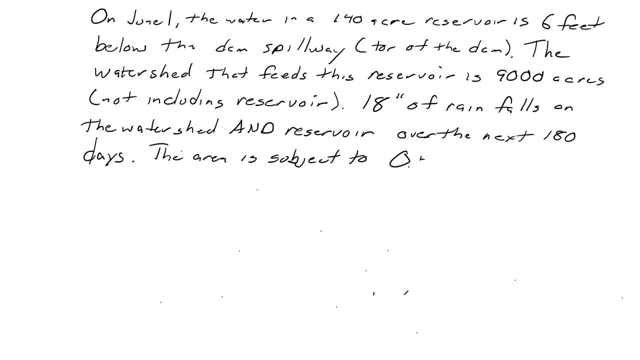 to half a centimeter of evaporation off the reservoir every day, which is a lot. Okay, a couple more things about this problem. The watershed is in the mountains And is largely unvegetated, With lots of exposed, unfractured granite. 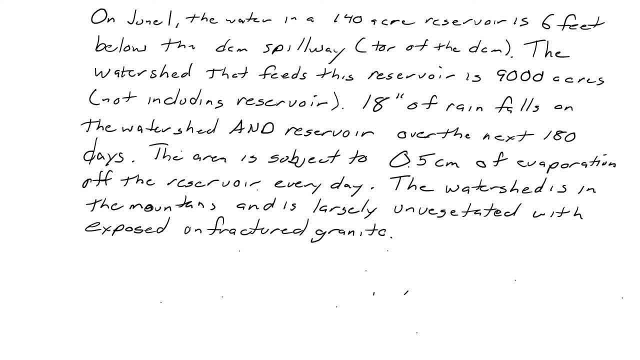 And because of this geology would you expect much infiltration into the ground. Why, or why not? Why not? The rock is, if you've seen granite, there's not much for pores right, And this is unfractured. 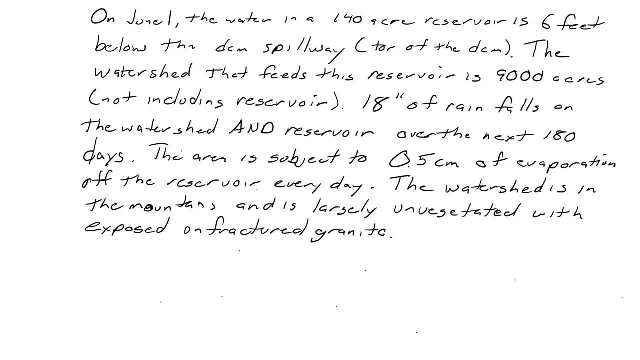 There's no plants, There's no trees, There's no plants, There's no rocks on it, It's just pretty much bare rock in the mountain. So rain's going to run and land on it and it's going to run off, right. 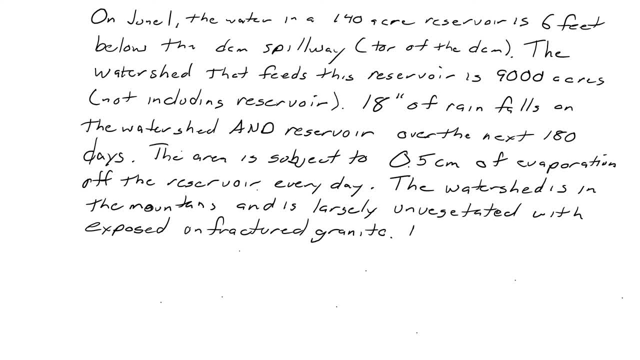 That's what's going to happen to most of it. Some will evaporate, Some will run off. So let me leave you with this. It is because of the geology expected that only 10% of the land is going to be affected. 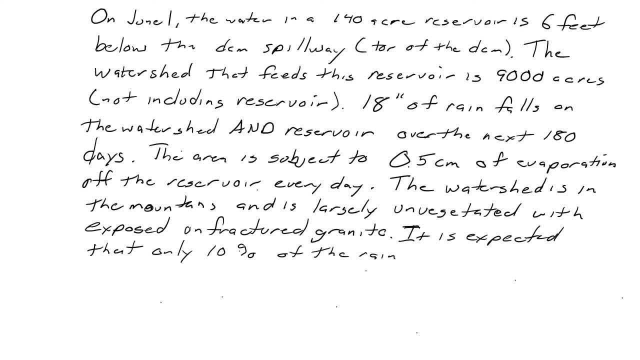 of the rainfall on the watershed will evaporate or infiltrate, So we're going to have to think about that. And that leaves 90% to runoff. And that leaves 90% to runoff. And that leaves 90% to runoff. 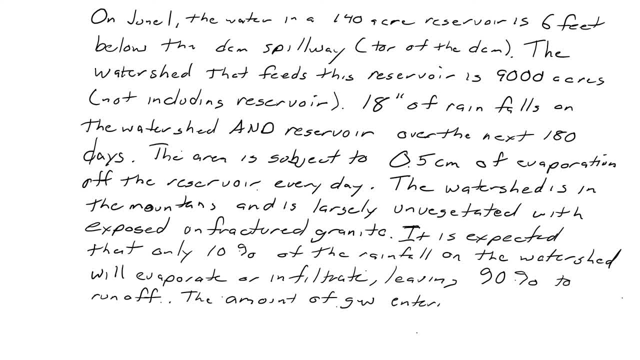 And finally, the amount of groundwater. the amount of groundwater entering or leaving, entering or leaving. and again The reservoir, because it's solid granite water's not going to move in or move out very easy. We're going to expect it to be negligible. 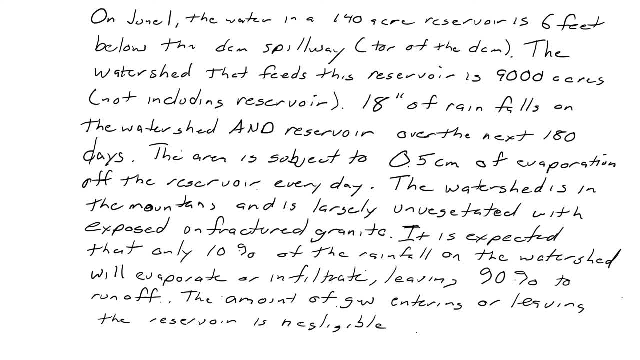 In other words, you can ignore it. Okay, so you have a dam. Behind the dam is a lake. It's six feet below the top. Over the next 180 days, 18 inches of rain is going to land. 90% of that is going to run off into the reservoir. 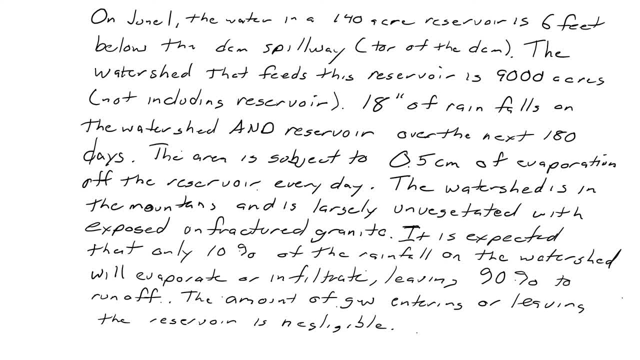 From a 9,000-acre watershed. If that was the only thing going on, what would happen to the level of the water? It would rise right, And as a dam manager, you'd want to know how high is it going to rise, right? 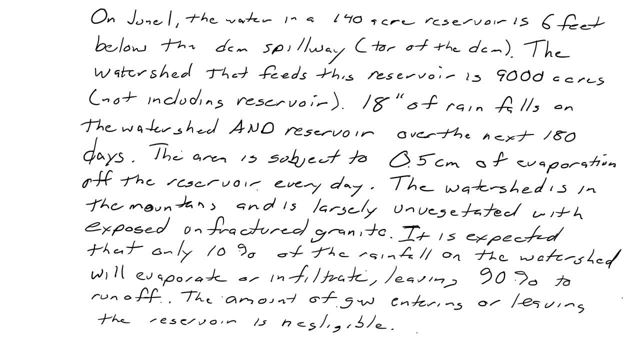 Because you don't want it to rise and overtop your dam, so you need to release some water. But what else has happened? That's not the only thing going on here. right, You have water leaving the dam right Through. primarily what? 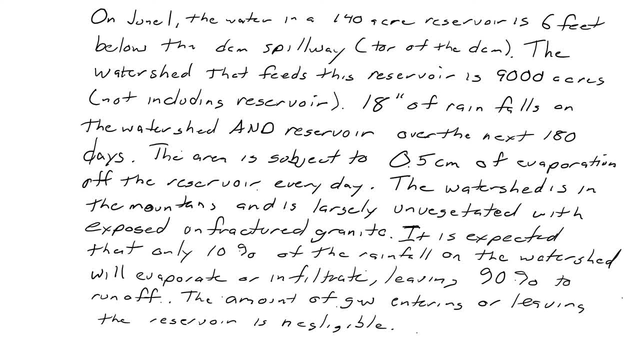 Evaporation. okay, So the question I have for you is: Let me change the color here. How much water, Yeah. How much water, Yeah. What is your dam singleton? Let me change the color to green, Let's see. 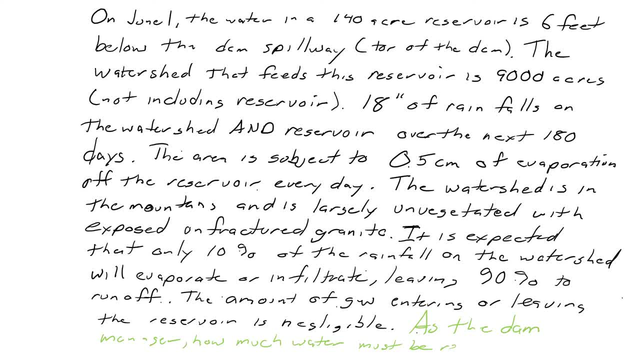 Yeah, green. Okay, let's make a question here. Yeah, Yeah, you had a water, чего? Yeah, If two levels are high, then does it go 하는데 water? Does it goorde and water? Yeah? 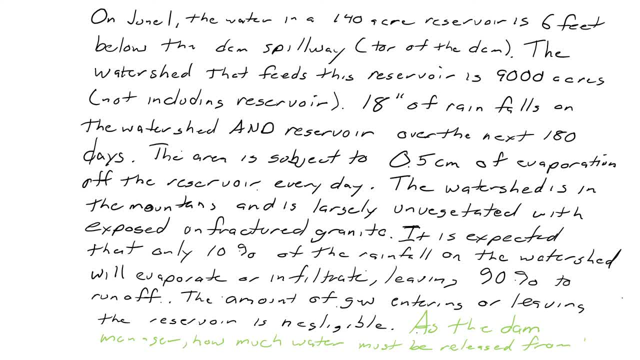 Absolutely must be released from the dam so that it doesn't overfill. Actually, let me change that part. As a dam manager, you never want it to get so close. Let's say your goal is to keep it at that six foot below the top level. 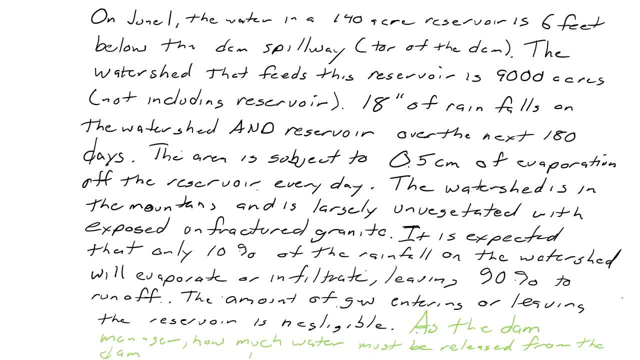 Let's go back to that. Let me just get rid of that question. I'm going to change that Dam so that it stays six feet below the top, or below the spillway, So that it stays there Or so that it just doesn't go over. 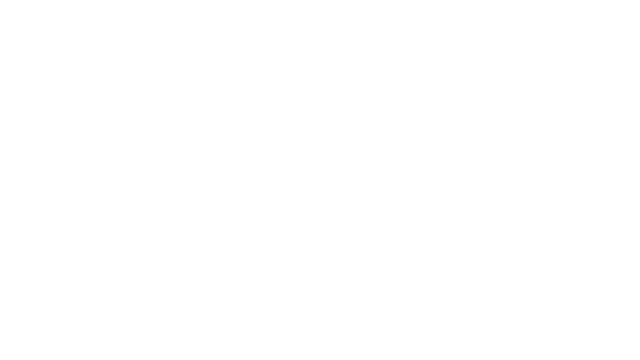 So by the end of the 180 days. Let me just go on to the next page here. Let's look at this from above. Let's see, Yeah, so let's say: this is our reservoir, Here's our dam, It's a map view. 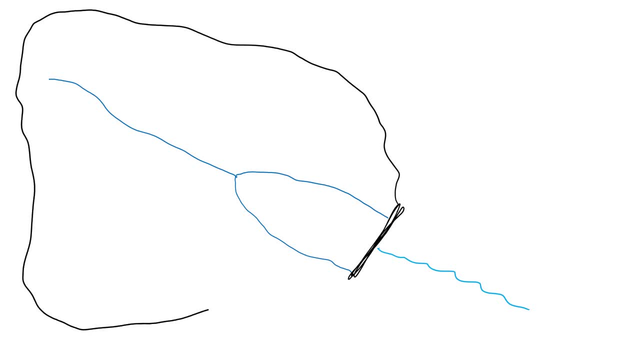 There's our outflow. This is not obviously going to be the scale, So this is our Okay. so this is the outline of the watershed. Remember it's 9,000 acres. Okay, Stream going in, Stream going out. 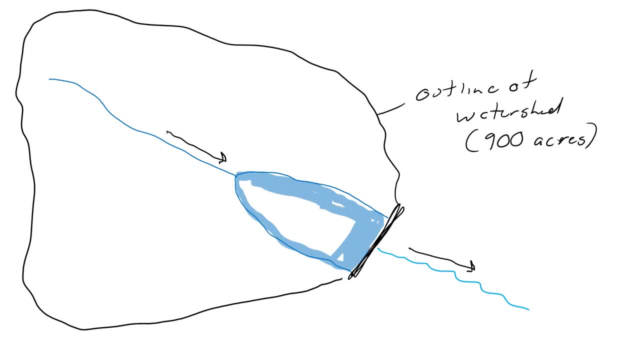 Here's your reservoir, which is 140 acres. no groundwater coming in or out. so after 180 days, 18 inches of rain are going to fall in the watershed, 90 is going to end up in the lake. you're going to get some evaporation. 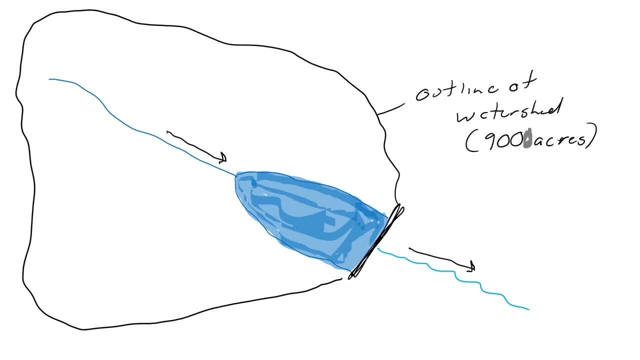 nine hundred thousand. thank you, yeah, those decimal points kind of matter okay. so the first thing that you do with these sorts of problems is identify all the inputs and outputs. okay now, one final bit here to sort of help you with this is: you see, we have a lot of water. you can't just let half the lake go in a second. 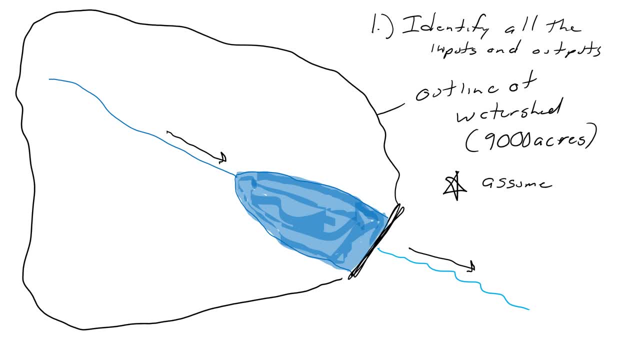 okay, it takes a long time to figure out. is this really happening? i want you to figure out. okay, as a dam manager, it takes time to let water go, right. you can't just let half the lake go in a second. okay, so you've got 180 days to let.